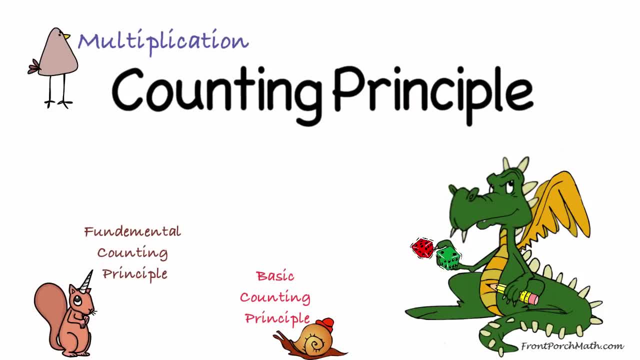 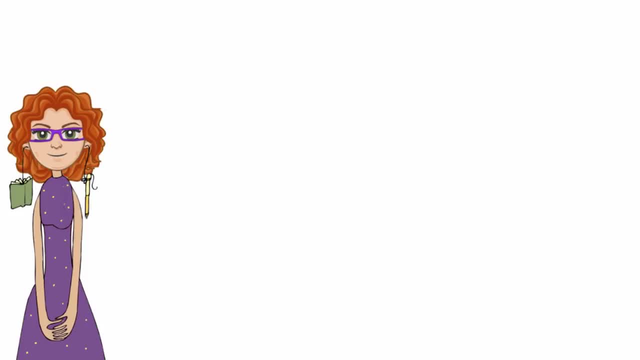 So today we're going to be learning about the counting principle. This is often used in probability and statistics to figure out how many possible options there are. So let's start with the situation that I bring my lunch to school every day. At home, I've got 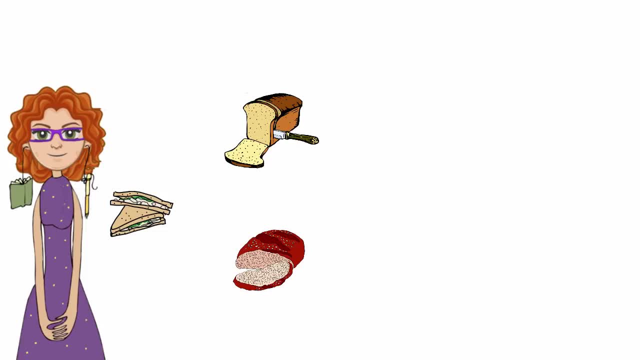 two types of bread: wheat bread and rye bread. I also have three types of fillings I like to use. I like tuna fish sandwiches, I like cheese sandwiches and I like peanut butter sandwiches. How many different combinations can I make so that I can have a different sandwich each day? 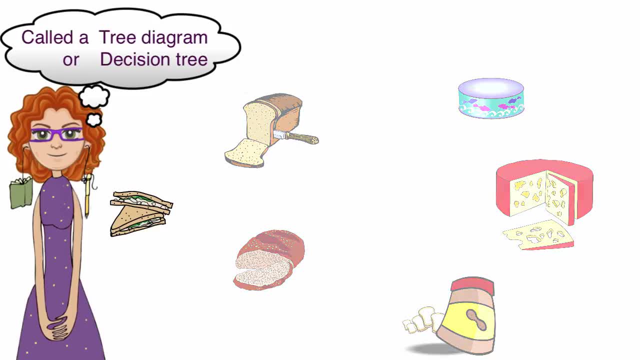 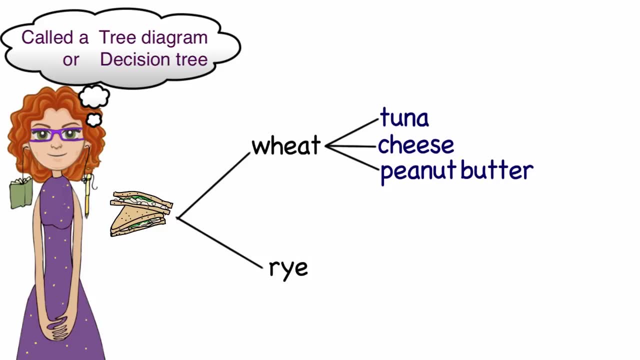 of the week. Well, one way to find that answer is to draw it out. I've got wheat and rye, and then for wheat I have the three options of tuna cheese or peanut butter, And for rye I have three options of tuna cheese and peanut butter, And we can see pretty quickly that we 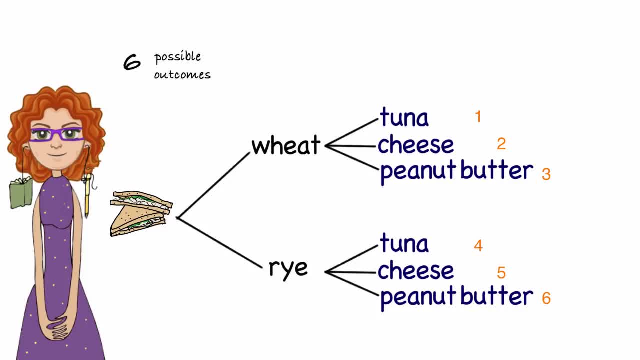 have six possible options. I can see there's a relationship between the number of decisions to be made and the possible outcomes. I could have multiplied two times three to find out that I had six possible options, And when I do that, I'm using the counting principle. The counting principle. 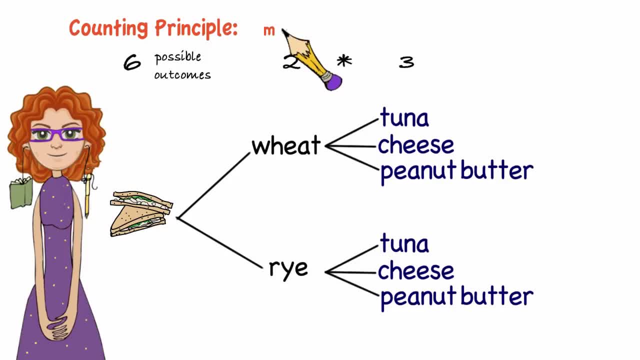 tells me that I have six possible options. I can see that I have six possible options. If we have two decisions to make and there are m ways to make the first decision and n ways to make the second decision, the product of m and n tells us how many different. 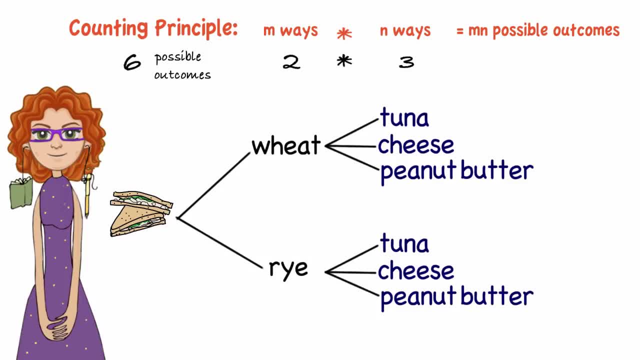 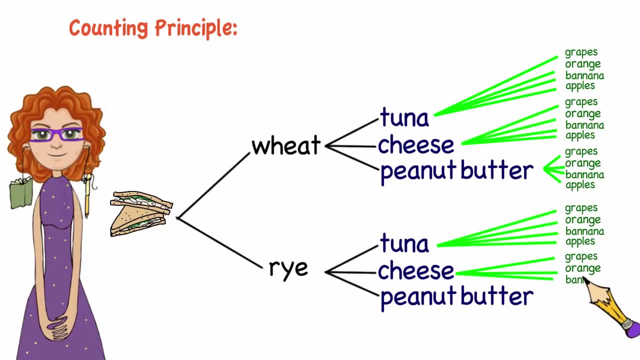 outcomes there are. So let's extend this example by adding one of four different fruits to my lunch. I happen to have grapes, oranges, bananas and apples at home. When I draw out the graph, you can see it becomes pretty cumbersome very quickly, And the more choices I have, the more complex. 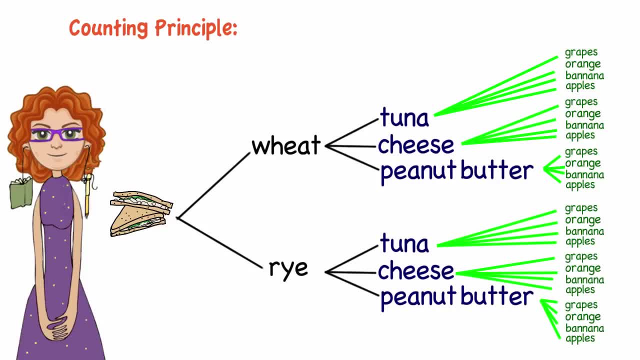 drawing it all out is: I can see that I have six possible options. I can see that I have six choices, But I can do it using the counting principle. By multiplying two times three times four, I can quickly see that I have 24 choices. And when we start looking at it in terms of 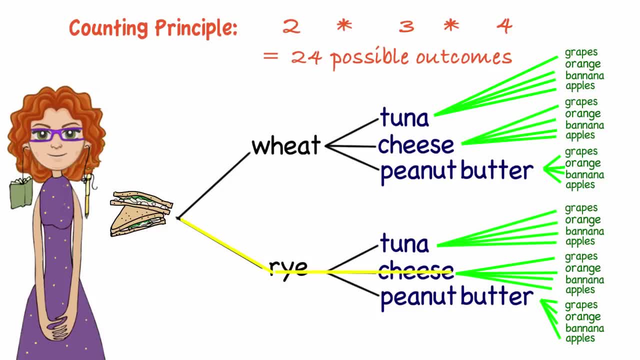 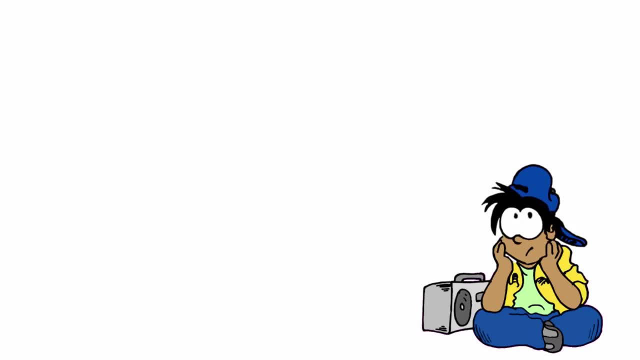 probability. I say: well, what is the chance? I'll pick any one of those by random. Well, that would be one in 24.. Let's look at another example. As of 2015, there are 15,330 US radio stations. 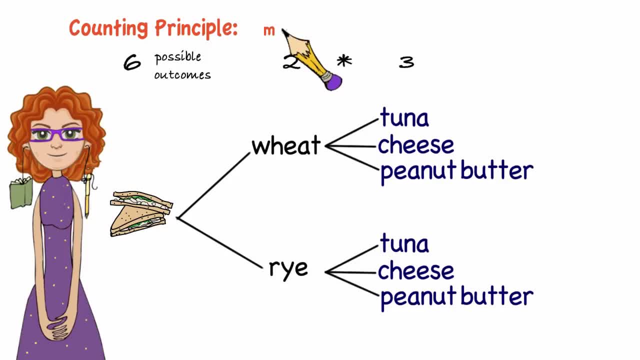 tells me that I have six possible options. I can see that I have six possible options. If we have two decisions to make and there are m ways to make the first decision and n ways to make the second decision, the product of m and n tells us how many different. 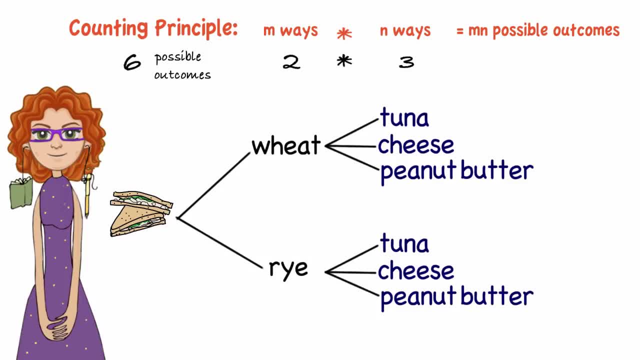 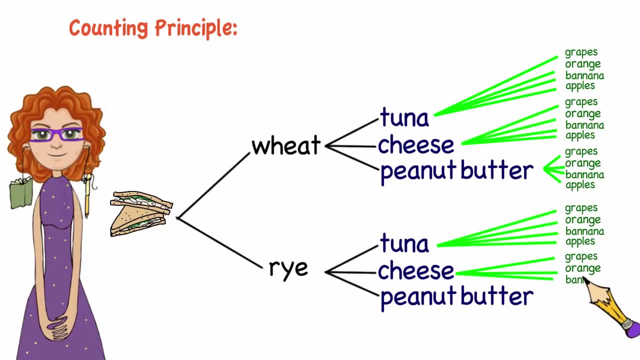 outcomes there are. So let's extend this example by adding one of four different fruits to my lunch. I happen to have grapes, oranges, bananas and apples at home. When I draw out the graph, you can see it becomes pretty cumbersome very quickly, And the more choices I have, the more complex. 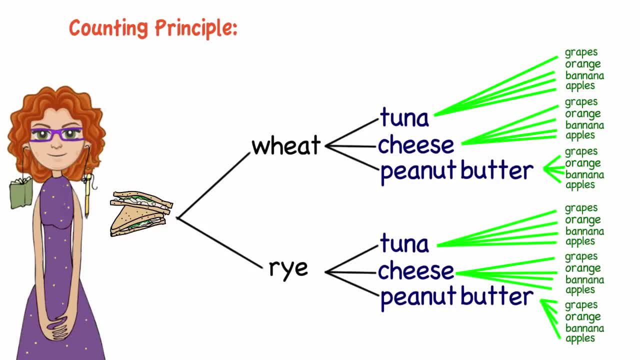 drawing it all out is: I can see that I have six possible options. I can see that I have six results, But I can do it using the counting principle. By multiplying 2 times 3 times 4,, I can quickly see that I have 24 choices. And when we start looking at in terms of probability, 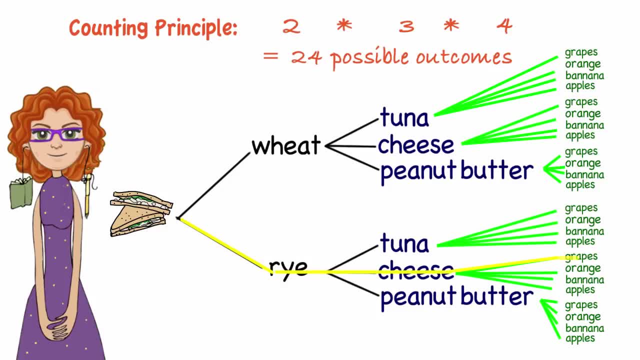 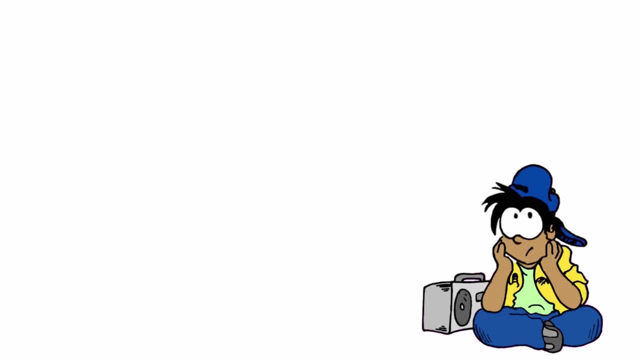 I say: well, what is the chance? I'll pick any one of those by random. Well, that would be 1 in 24.. Let's look at another example. As of 2015,, there are 15,330 US radio stations. 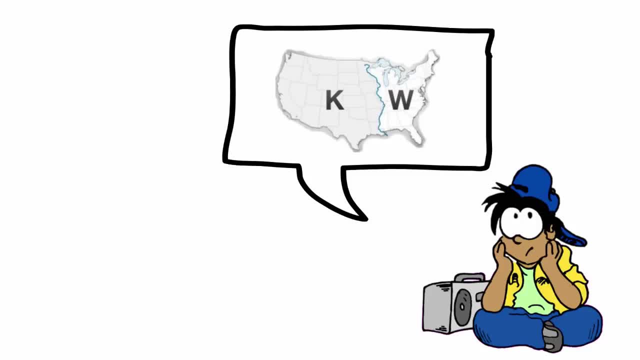 Radio stations must start with the letter W or K, depending on where you live. How many four-letter combinations can there be so that each station will have its own call letters? One way of doing that is to lay out my four possible options. Well, I know. the first letter has to be either a W or a K. 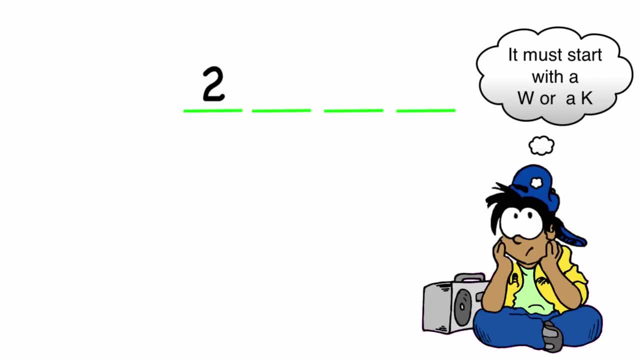 so I have two options. so I'll put a 2 in the first space, Then the next letter can be any one of the 26 letters in the alphabet, so I'll have 26 there. There are also 26 options for the third letter and 26 options for the fourth letter. 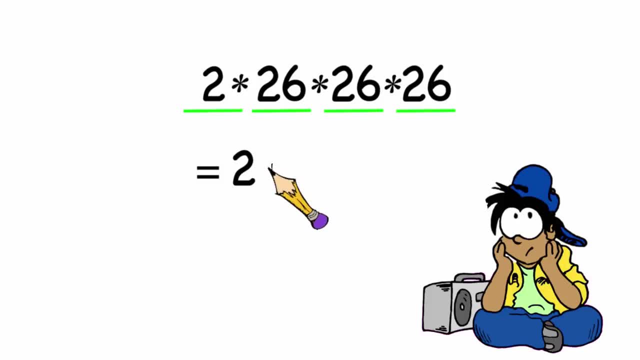 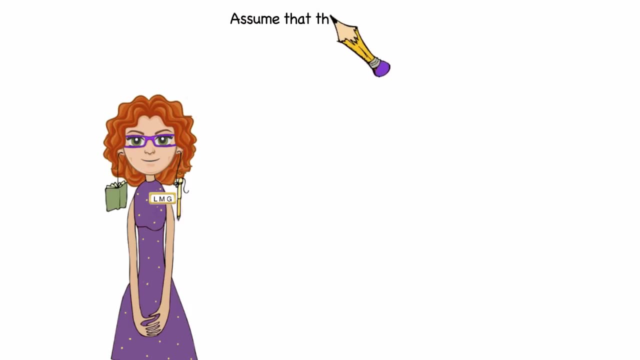 By using my counting principle, I can say that answer is 2 times 26 to the third power, or 35,152 possible combinations. Okay, let's look at a third example. Let's assume that there are roughly 300 million people in the United States. 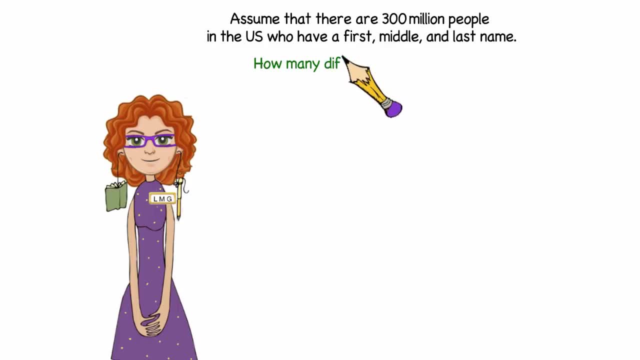 that have a first, a middle and a last name. So how many different three-letter combinations of initials are there? Well, it's very similar to the other question. We have three possible options and there's 26 letters for the first choice. 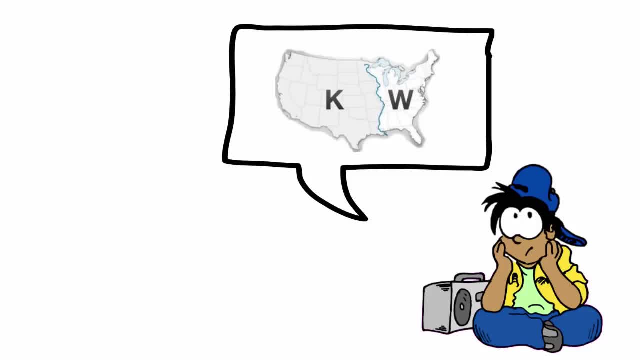 Radio stations must start with the letter W or K, depending on where you live. How many four-letter combinations can there be so that each station will have its own call letters? One way of doing that is to lay out my four possible options. Well, I know. the first letter has to be either a W or a K. 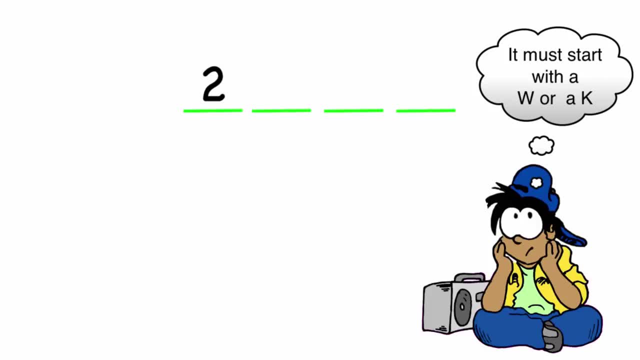 so I have two options. so I'll put a 2 in the first space, Then the next letter can be any one of the 26 letters in the alphabet, so I'll have 26 there. There are also 26 options for the third letter and 26 options for the fourth letter By using my. 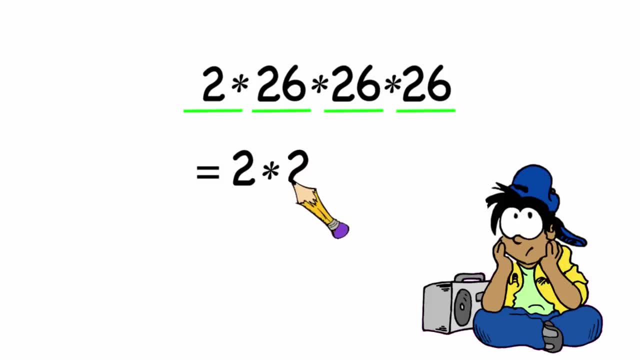 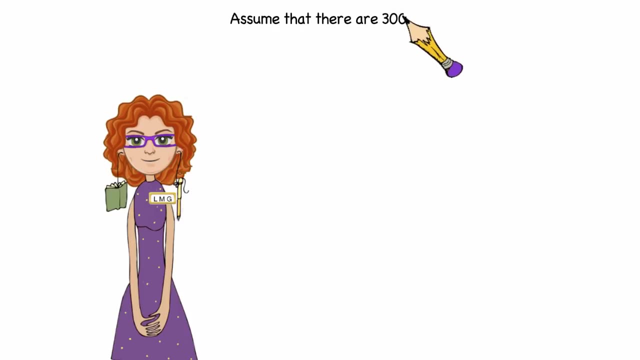 counting principle, I can say that answer is 2 times 26 to the third power, or 35,152 possible combinations. Okay, let's look at a third example. Let's assume that there are roughly 300 million people in the United States that have a first, a middle and a last name. So how many different? 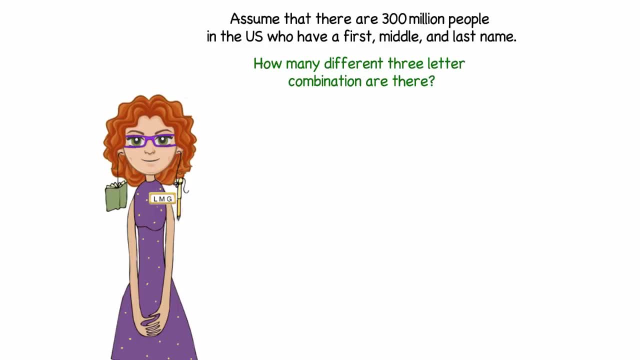 three-letter combinations of initials are there. Well, it's very similar to the other question. We have three possible options and there's 26 letters for the first choice, 26 for the second and 26 for the third. So when I multiply that out, I get 26 to the third power, or 17,576.. If we assume that, 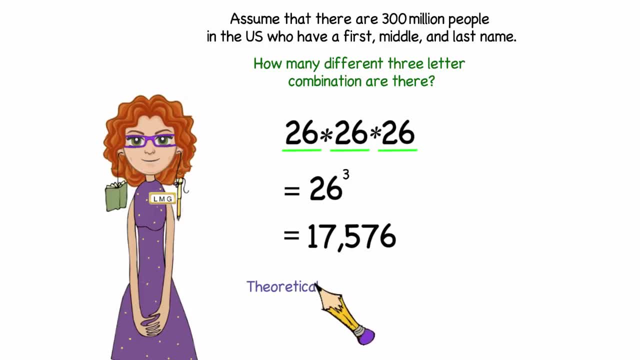 all possible three-letter initials are equally likely. what is the probability that someone will have my initials LMG? Well, that would be 1 out of 17,576.. And about how many people in the United States would you expect to have initials LMG? Well, that. 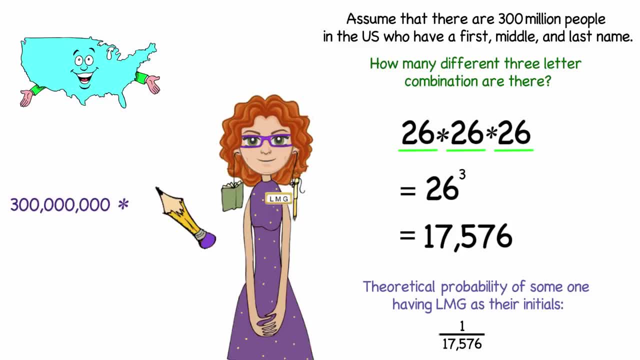 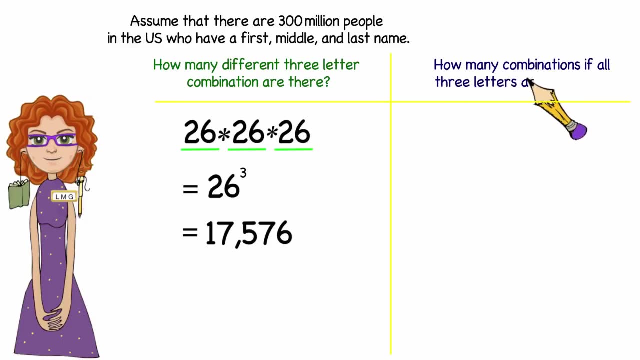 would be approximately the 300 million times the probability of my letters, and when I multiply those together I get 17,169 people. What if I change that problem a little bit? What if I want to know how many possible combinations where all three letters are different? Well, 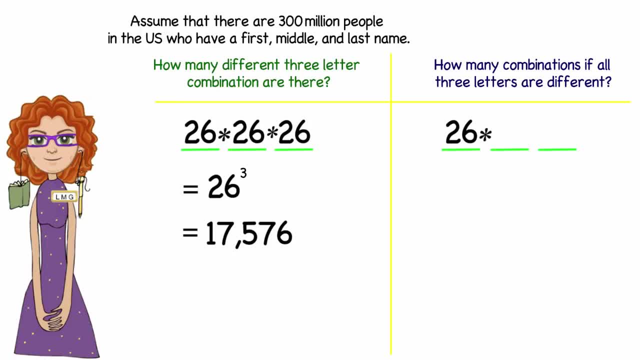 there'd be 26 for the first letter option, but I've used up a letter, so now there's a total of 25 for the second option and 24 for the third option And I would need to multiply those out to find out the total. So that would be 26 times 25 times 24 or 15,600.. The counting principle or